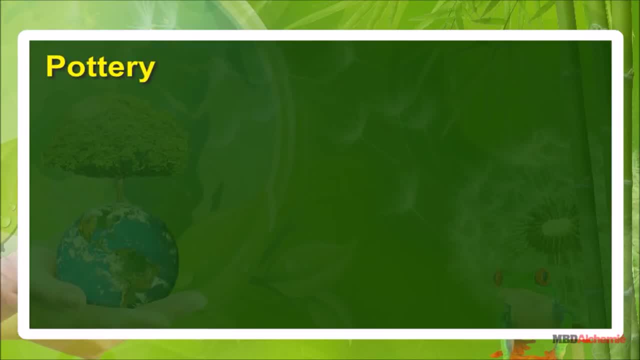 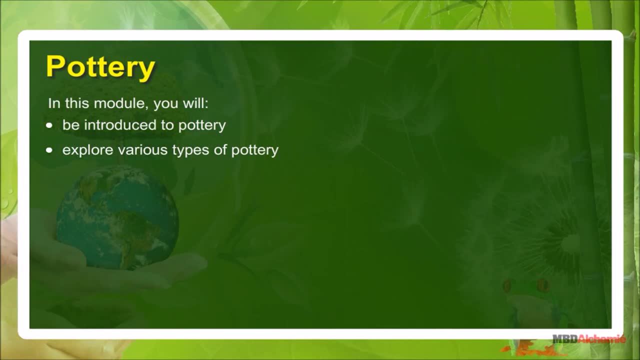 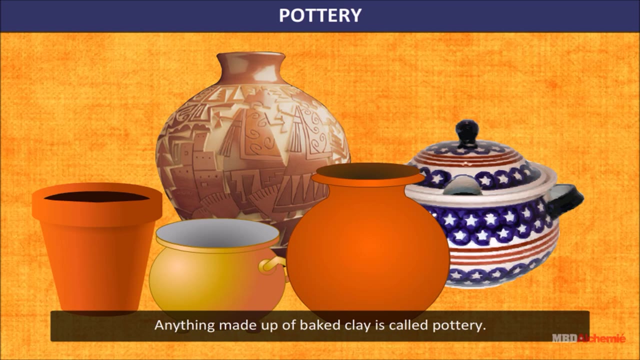 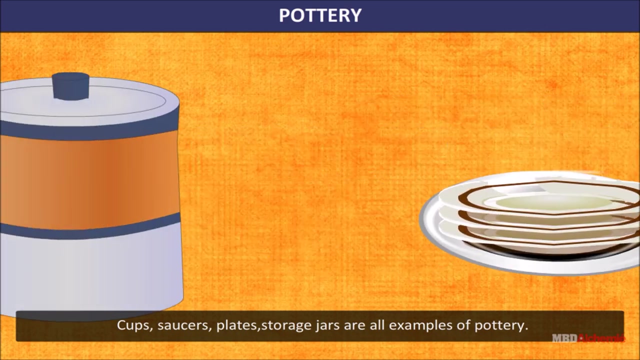 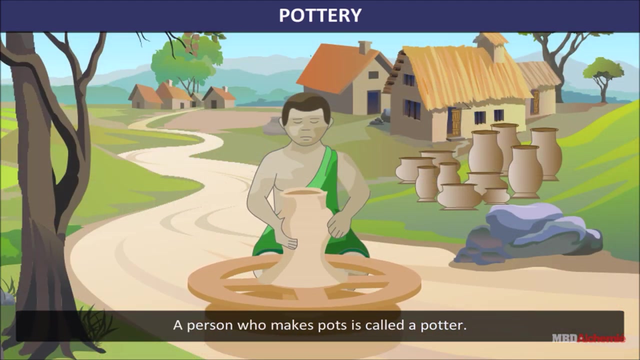 Pottery. In this module, you will be introduced to pottery and explore various types of pottery Pottery. Anything made up of baked clay is called pottery. Cups, saucers, plates, storage jars are all examples of pottery Pottery. A person who makes pots is called a potter. 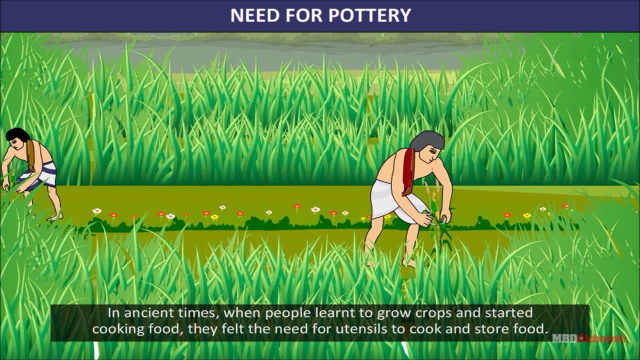 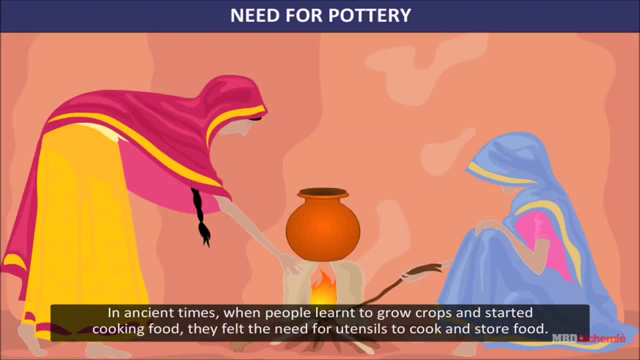 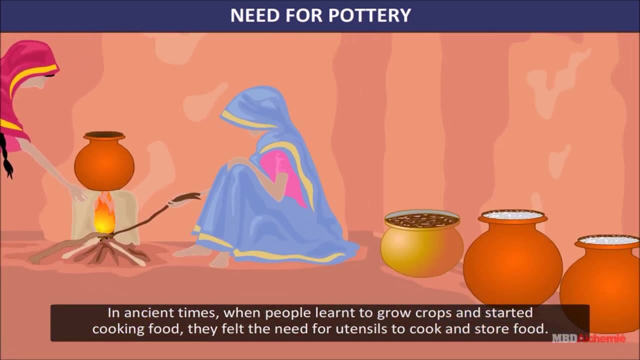 Need for Pottery. In ancient times, when people learnt to grow crops and started cooking food, they felt the need for utensils to cook and store food. Earlier, they used coconut shells and big leaves As means of storing food. Then they learnt to make pots with clay. 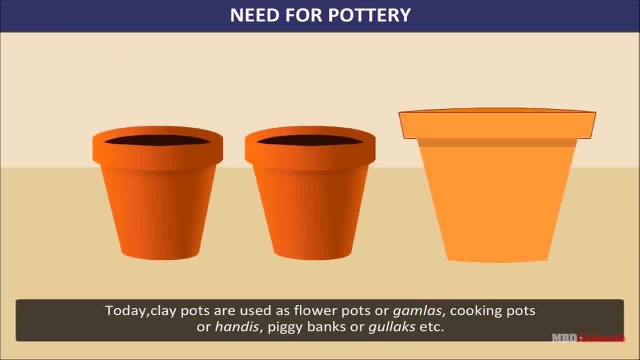 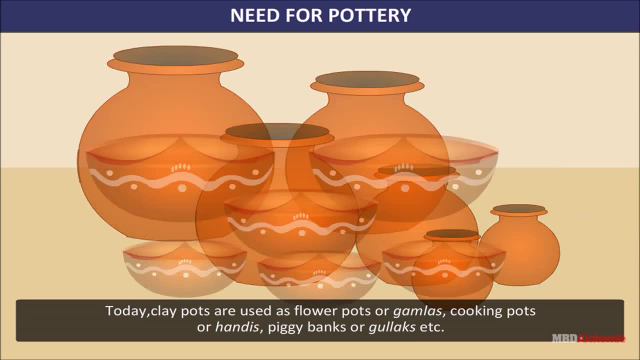 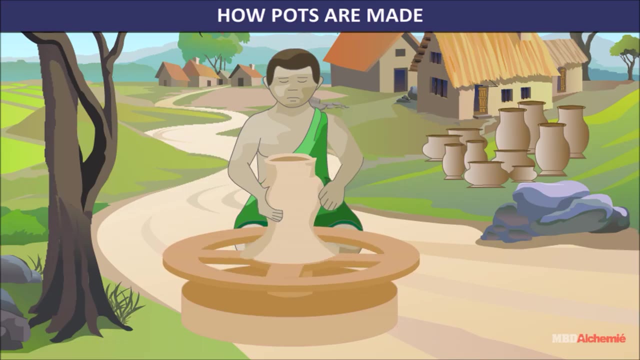 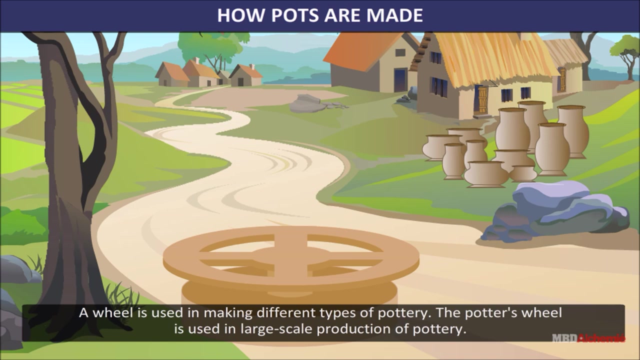 Today, clay pots are used as flower pots or gamlas cooking pots or handis, diyas, piggy banks or gulags, etc. How Pots are Made. First, a wheel is used in making different types of pottery. The potter's wheel is used in large-scale production of pottery. 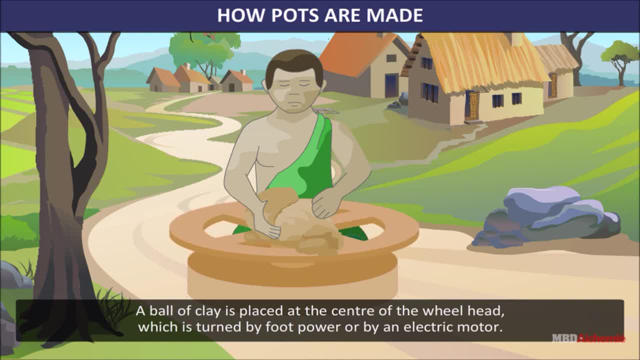 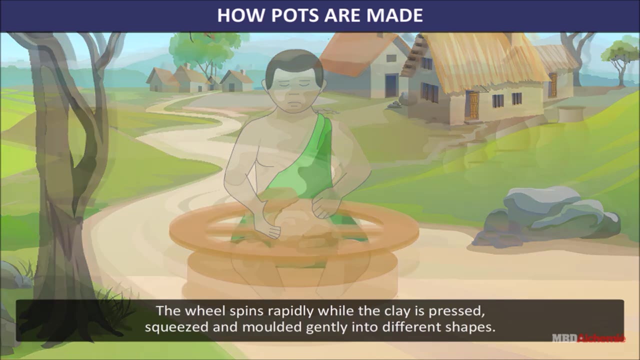 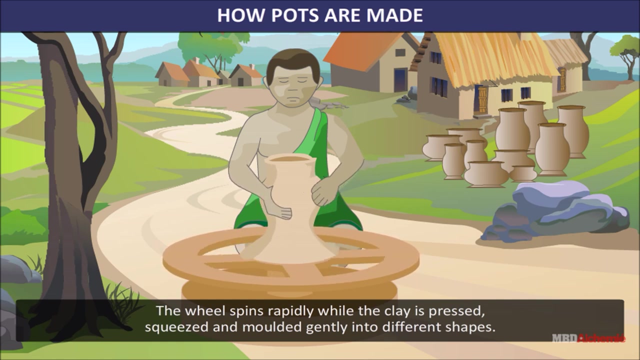 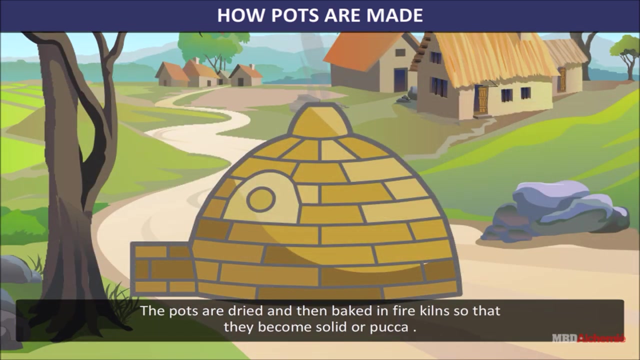 A ball of clay is placed at the centre of the wheel head, which is turned by foot power or by an electric motor. The wheel spins rapidly While the clay is pressed, squeezed and moulded gently into different shapes. The pots are dried and then baked in fire kilns so that they become solid or pakka. 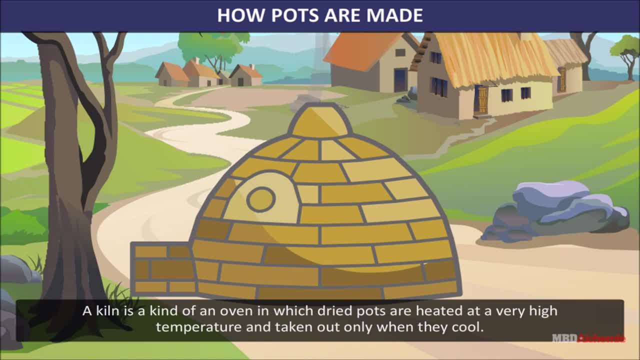 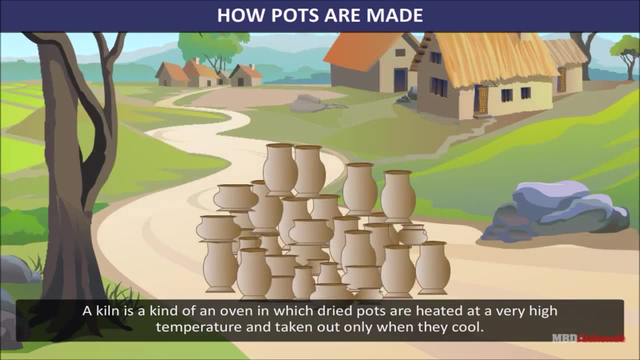 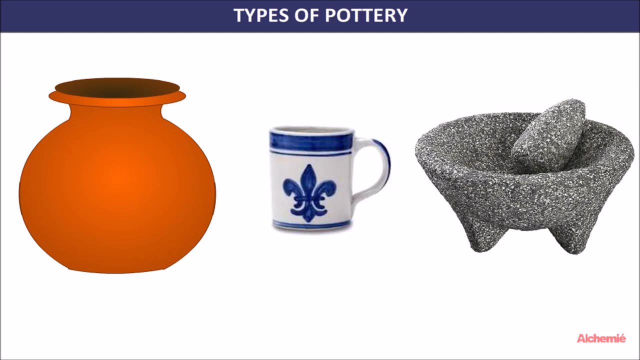 A kiln is a kind of an oven in which dried pots are heated at a very high temperature. Then the pot is passed out of the kiln and taken out only when they cool. Types of Pottery. There are three major types of pottery.